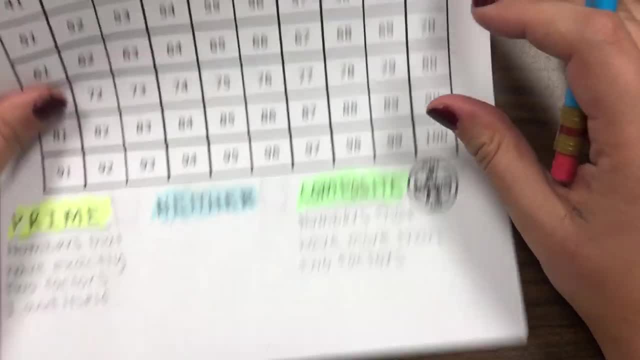 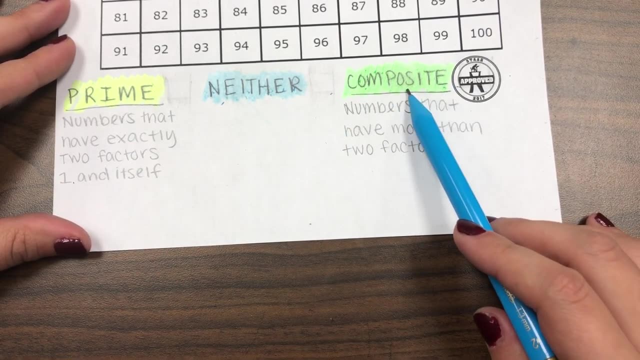 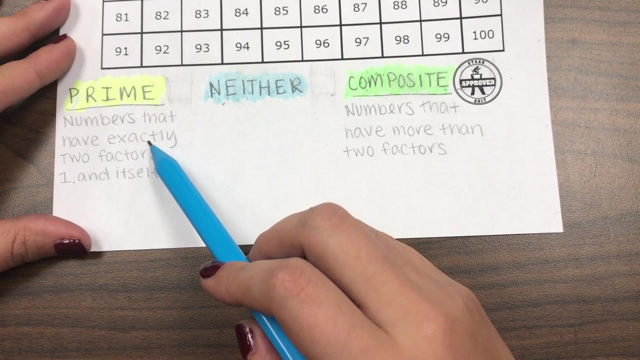 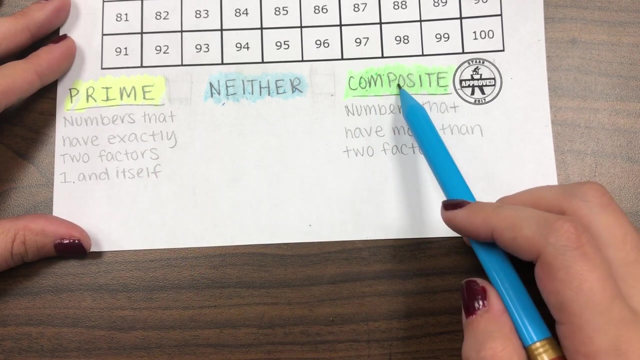 chart and down at the bottom I went ahead and labeled prime, neither and composite- okay. So prime numbers are numbers that have exactly two factors: one and itself- okay, And a composite number is a number that has more than two factors. 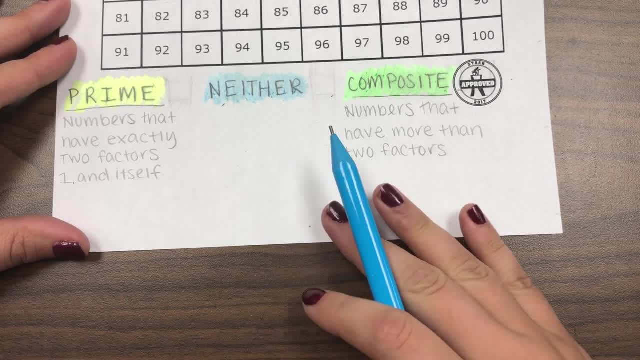 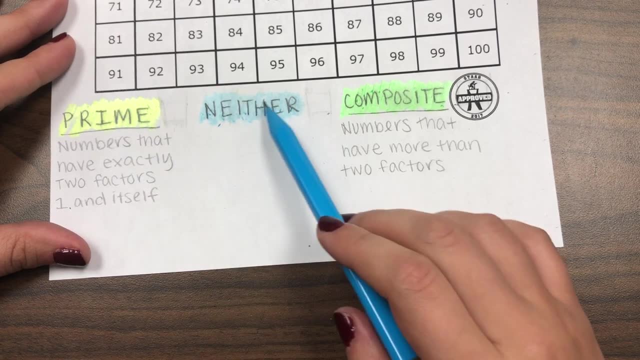 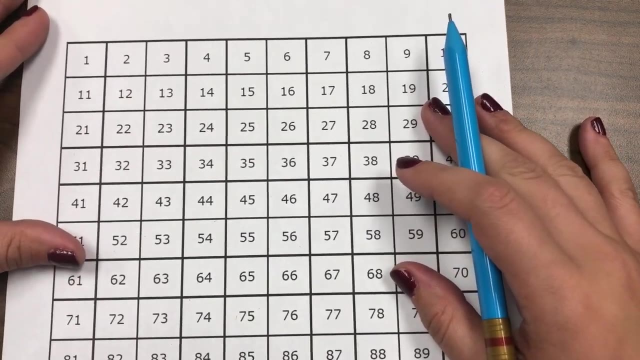 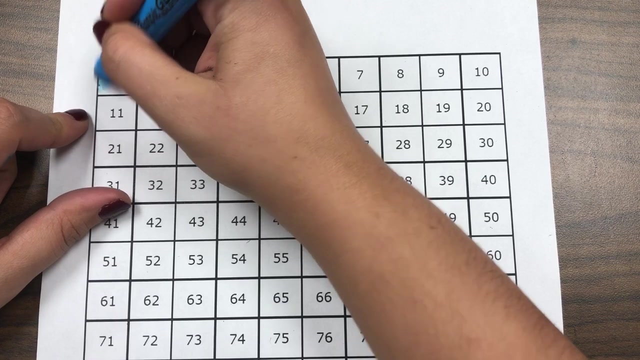 Okay, and I'm gonna show you what that means in a minute. okay, So we're going to be using three colors. okay, I used yellow, blue and green. okay, And we're gonna start with blue. So the number one is going to be colored blue because the 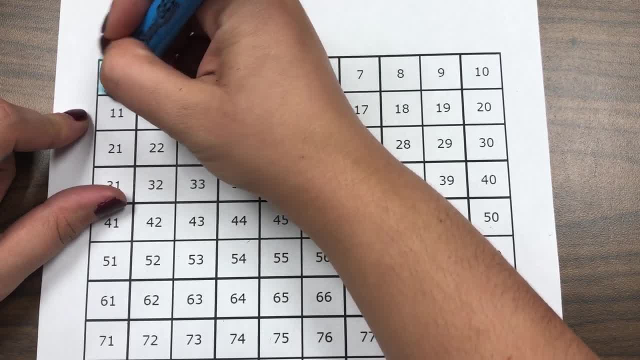 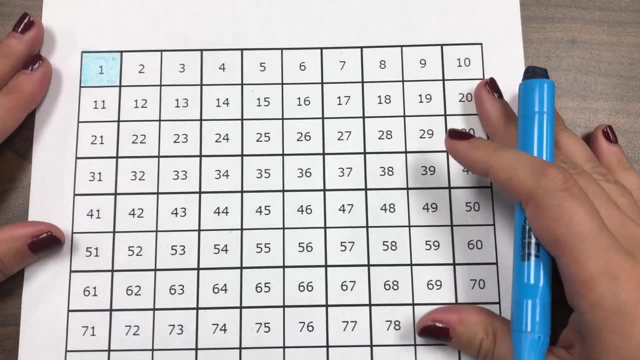 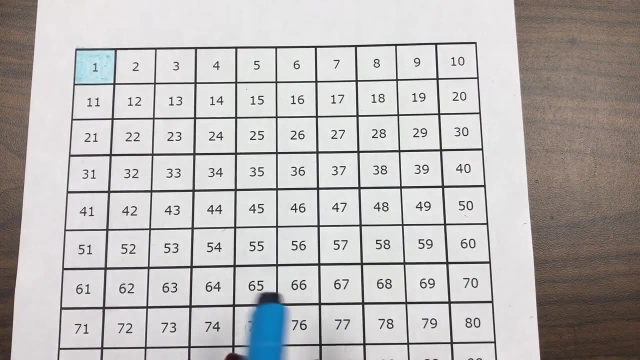 number one is the only number in the entire world- world that is not prime and it's not composite- okay, it is neither. it's independent. all by itself, it's very special, okay. now what we're gonna be doing is we're going to be skip counting by two, three and five. okay, so we're. 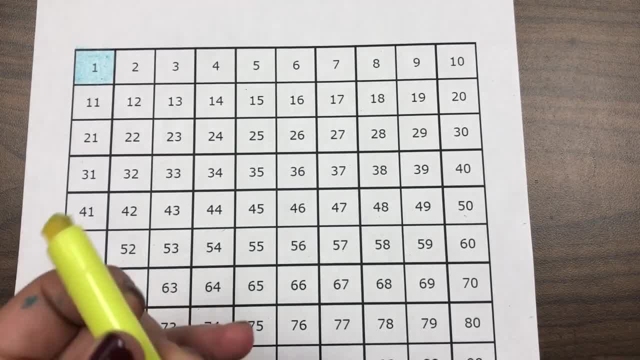 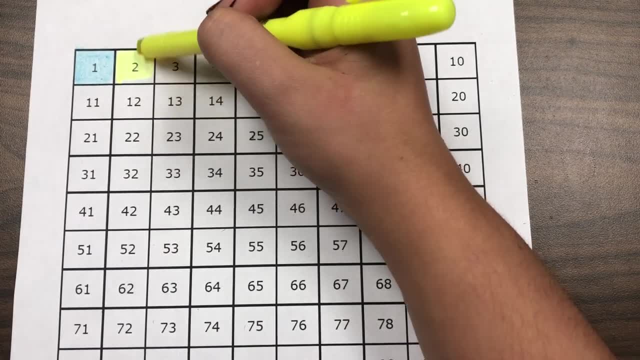 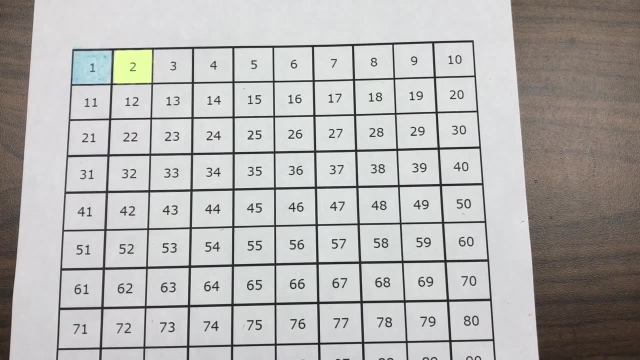 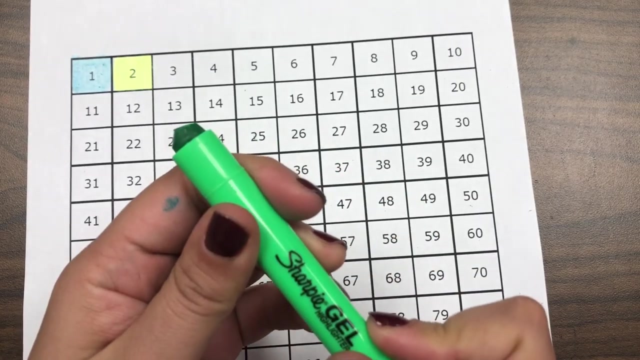 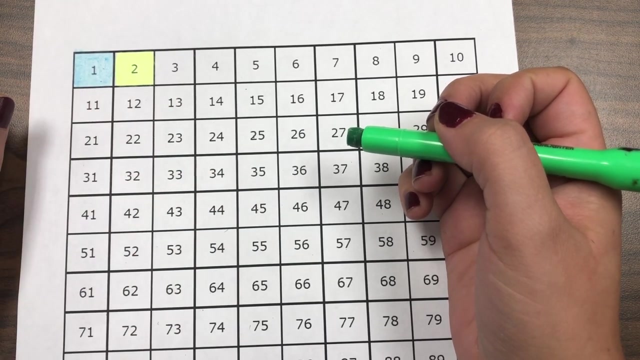 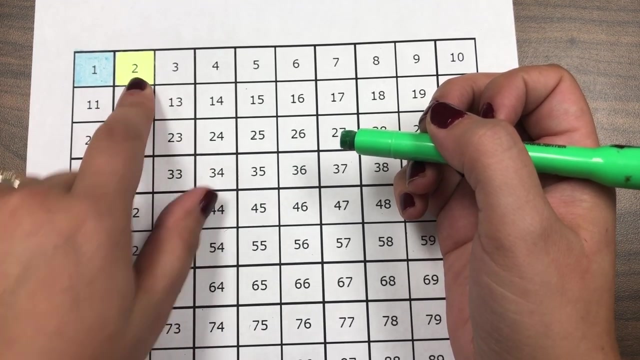 gonna start with two, so the number two is the very first prime number. so we're gonna color that number yellow. okay, now, from here we're gonna get our green and we're gonna use our green marker to color our all of the multiples of two, or we're gonna be skip counting by two. okay, so two. 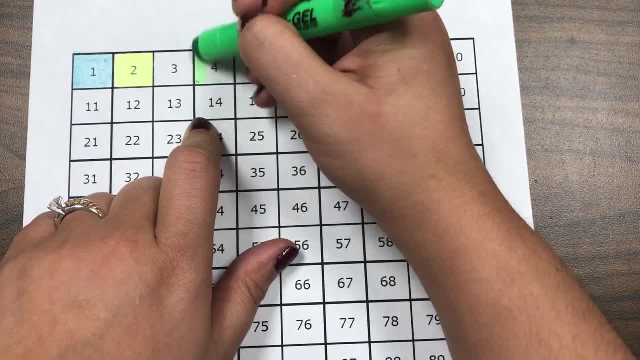 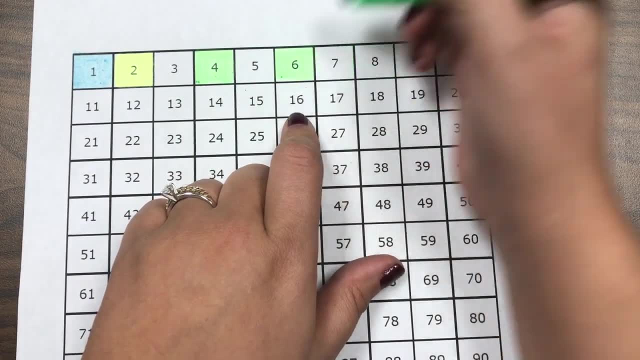 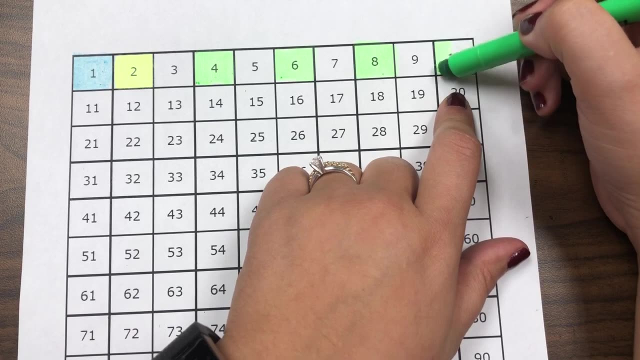 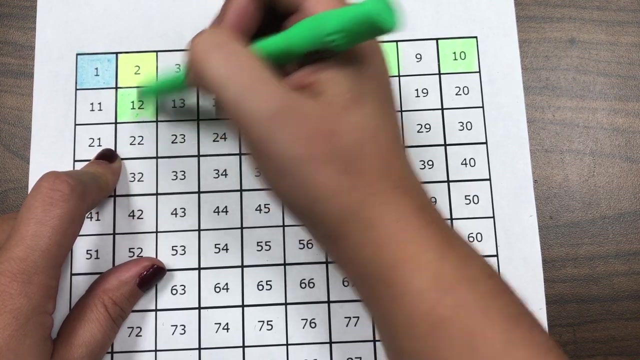 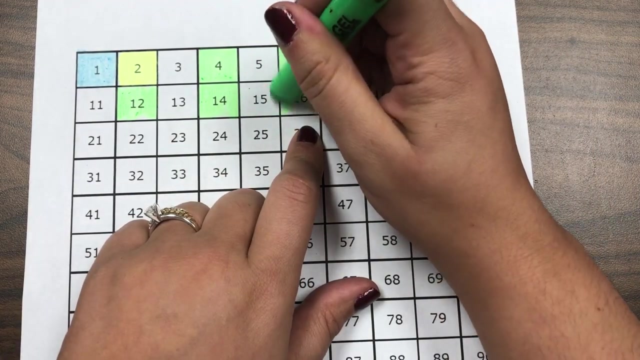 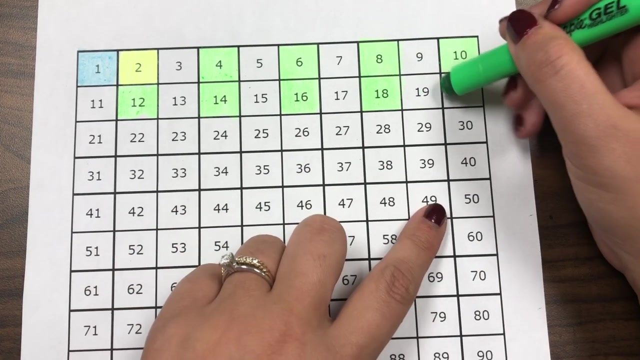 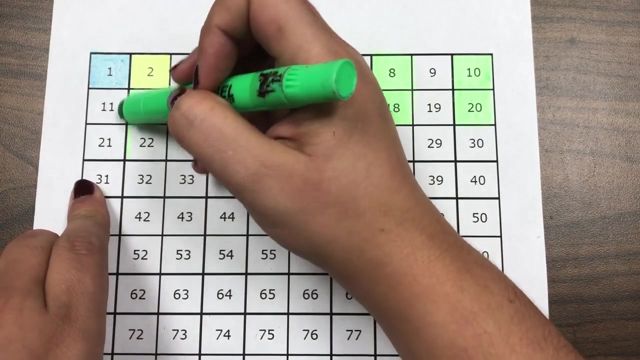 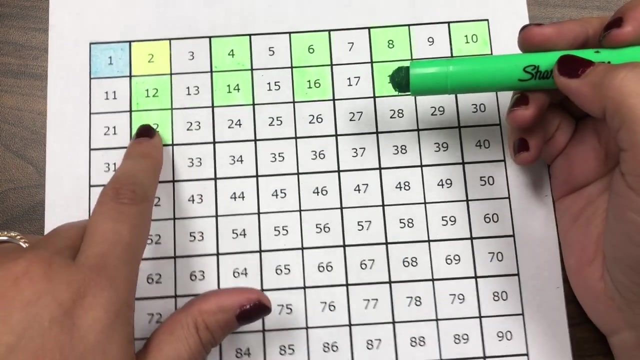 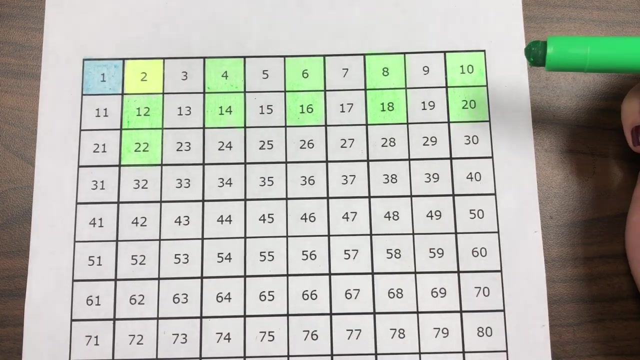 and then we're gonna go to four, and then we're gonna go to six, eight, ten, twelve, fourteen, sixteen, eighteen, 20. now here you should start to notice a pattern. if you notice, we are going to be coloring every other column. okay, the columns are the ones that go straight down, so all of the numbers that end. 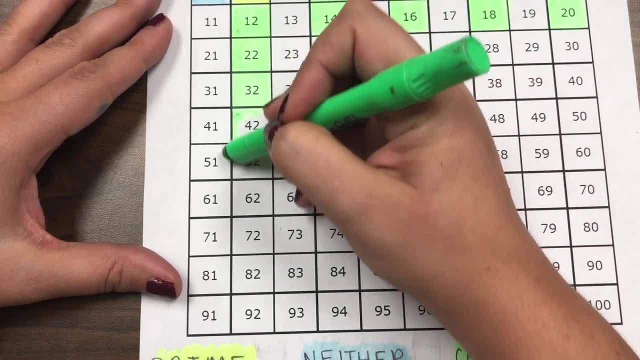 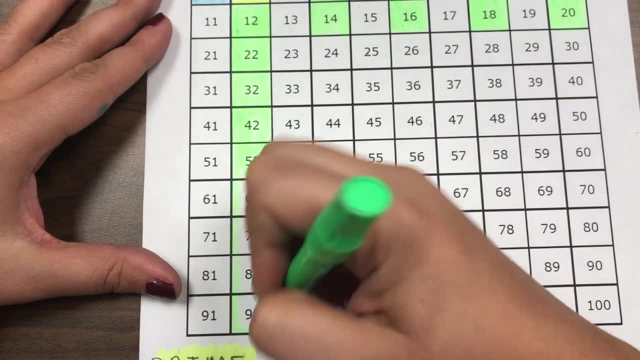 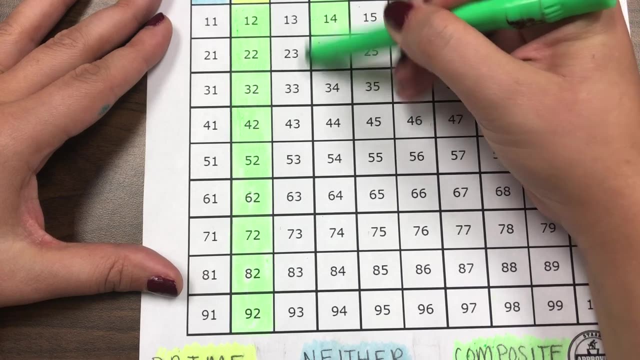 in an even number like two. all of these have a two at the end, so all of these are even so. we're gonna color all of those. then all of these have a four at the end. that means it's also even so. we're gonna color all of these. 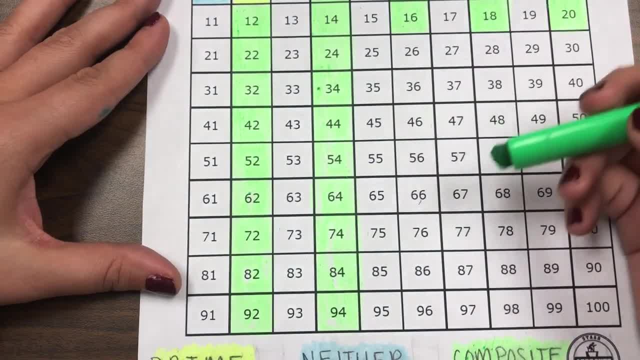 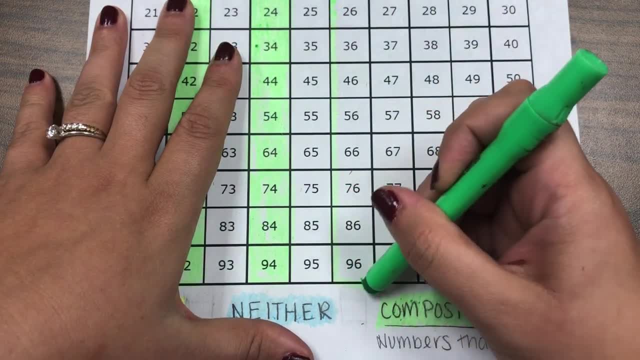 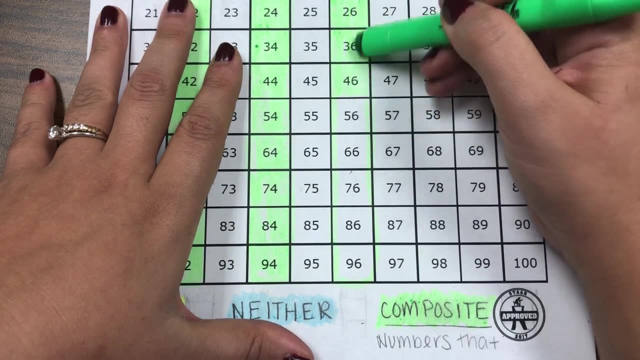 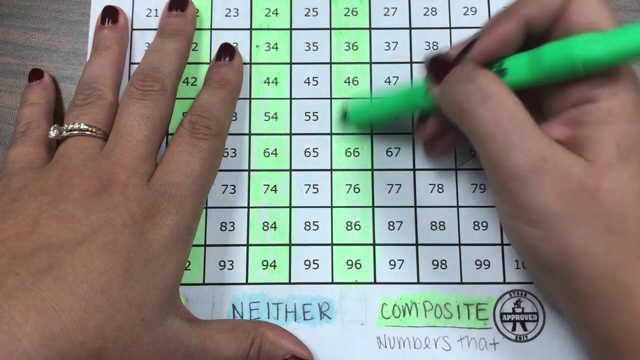 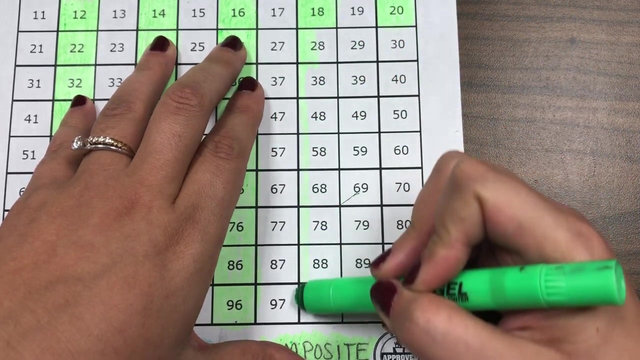 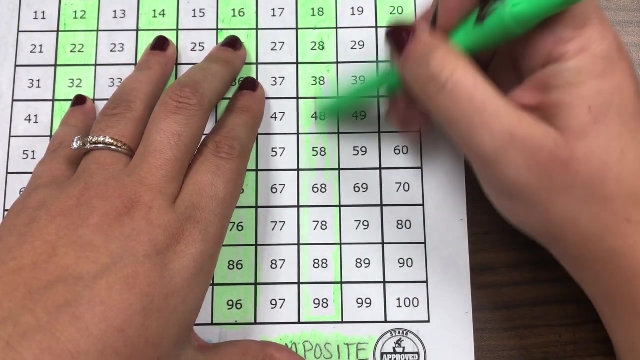 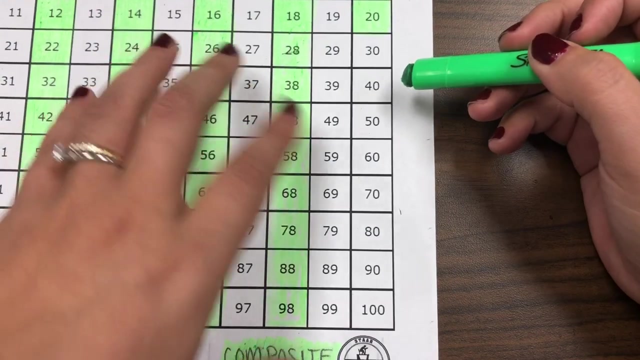 all of these have a six at the end, so we're gonna color all of these. all of these have an eight at the end, so we're gonna color all of these. and all of these have a zero at the end, so we're gonna color all of these two. 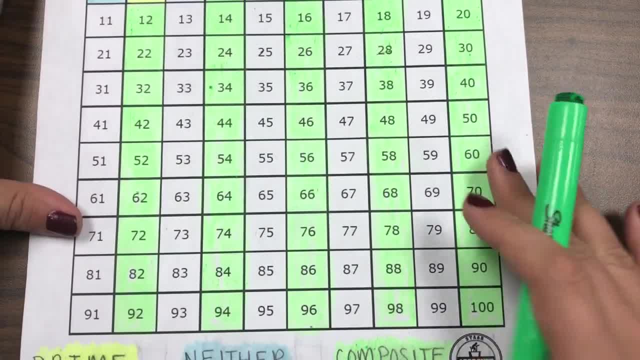 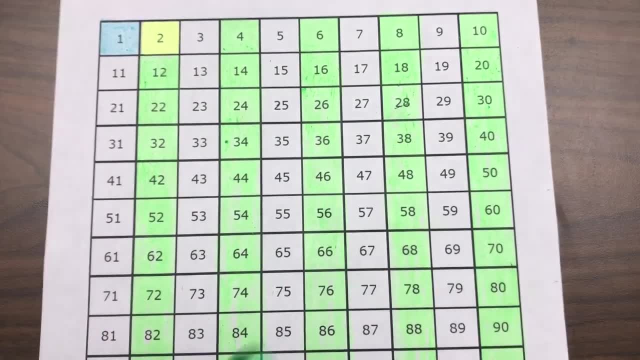 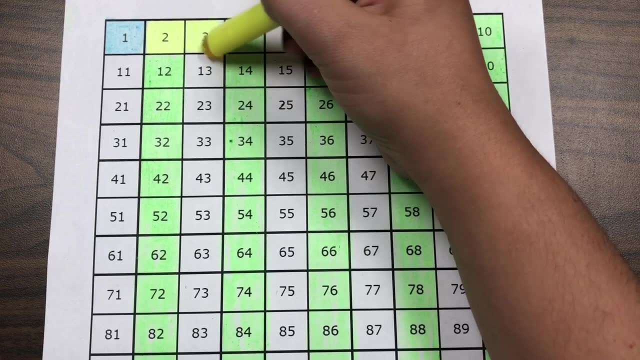 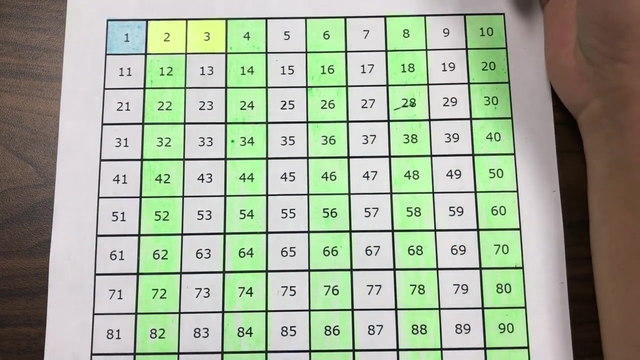 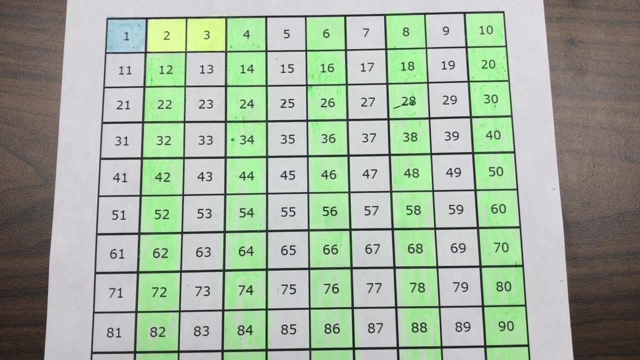 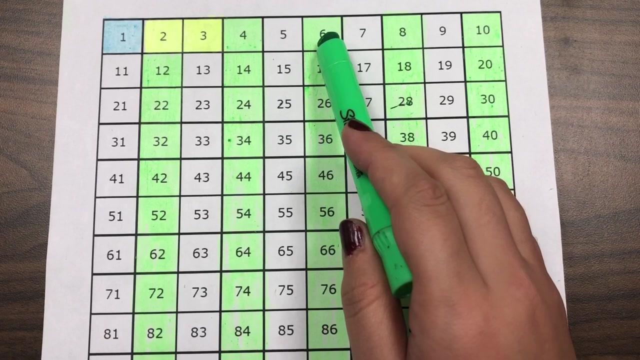 okay, so half of our hundreds chart is already colored. now we're gonna go to our second prime number, and the second prime number is three. so we're going to color that yellow because it's prime. now, guess what we're gonna do? we're going to count or skip, count by threes. okay, so three, six. oh, that's already colored. 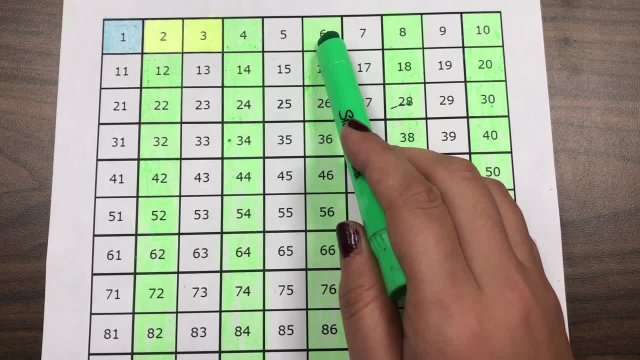 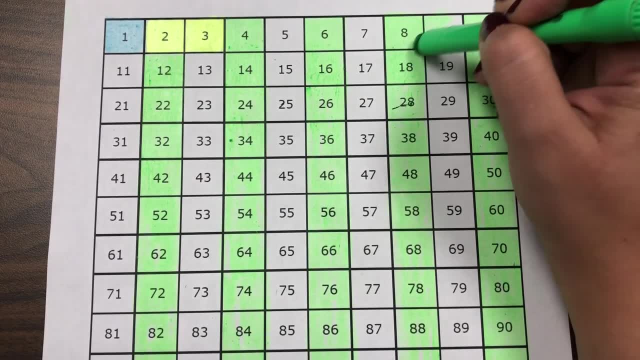 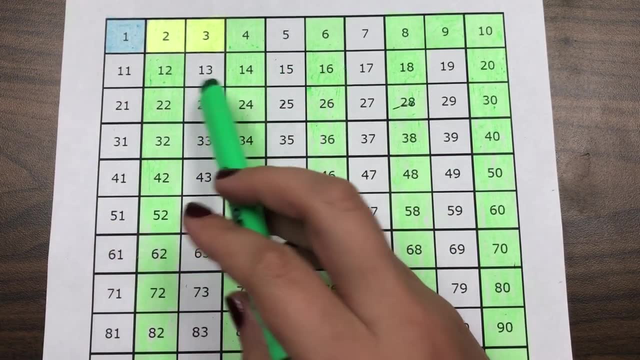 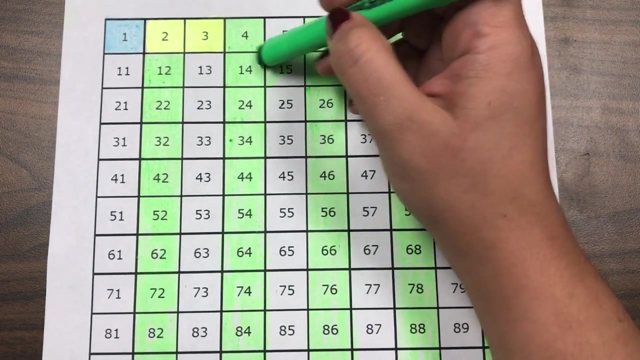 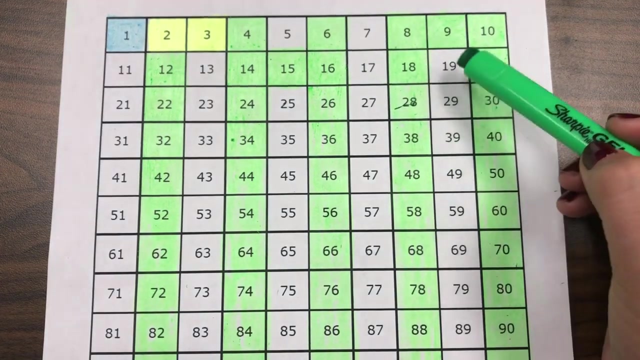 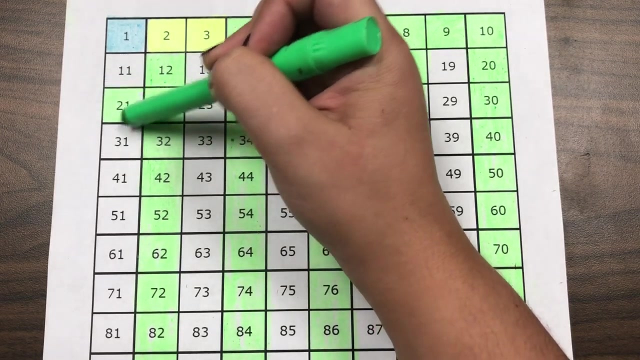 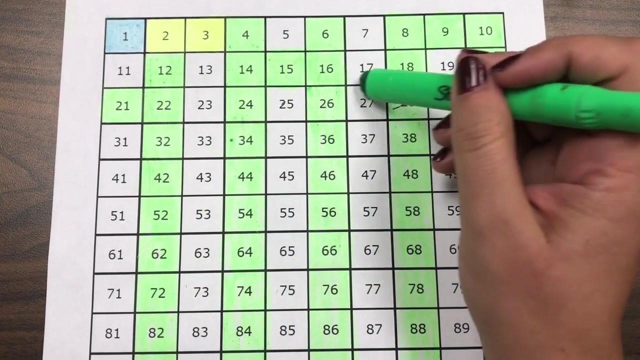 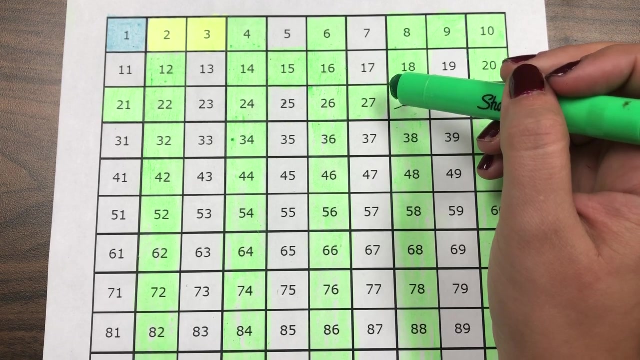 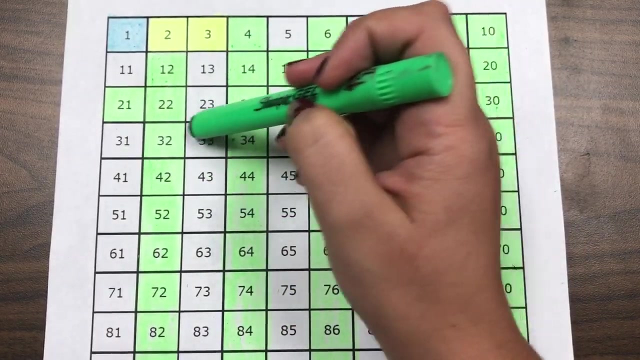 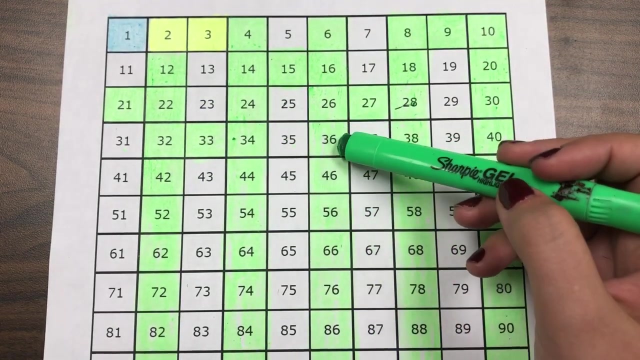 because it was also a multiple of two, nine. nine is not colored, so we're gonna color that one. 12, 15, so we're gonna call her 15, 18, 21, 24, 28- I'm sorry- 27, 30, 33, 36, 39. 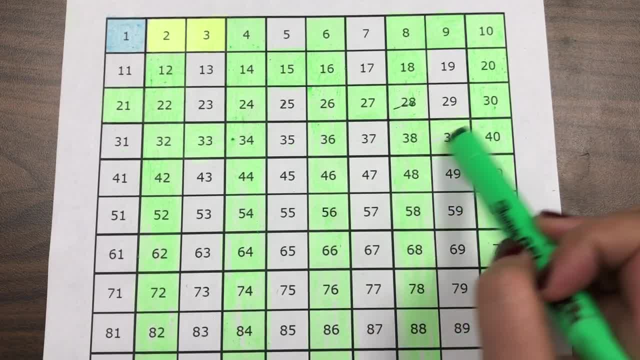 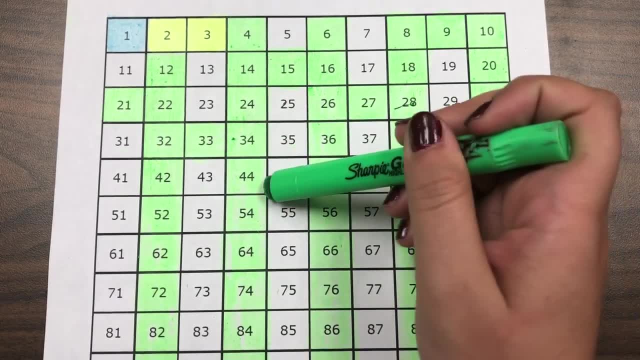 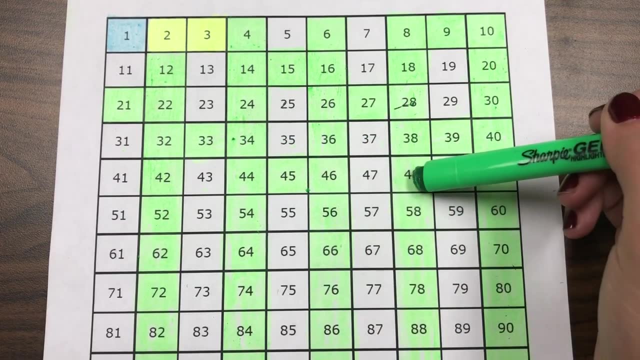 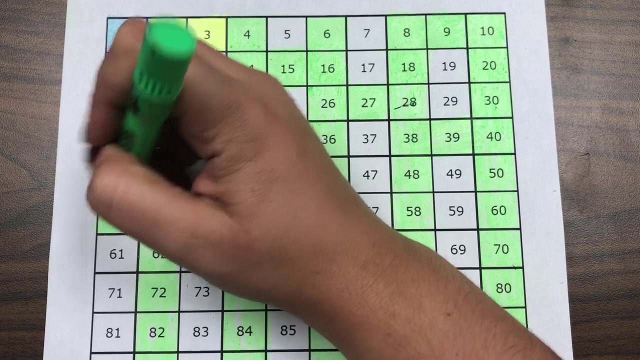 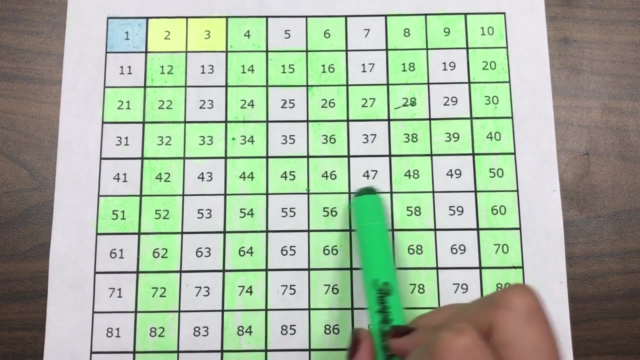 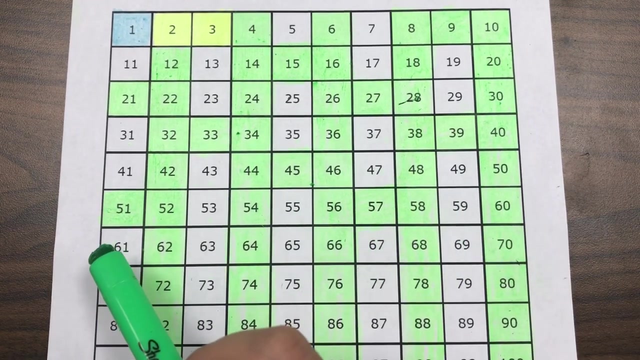 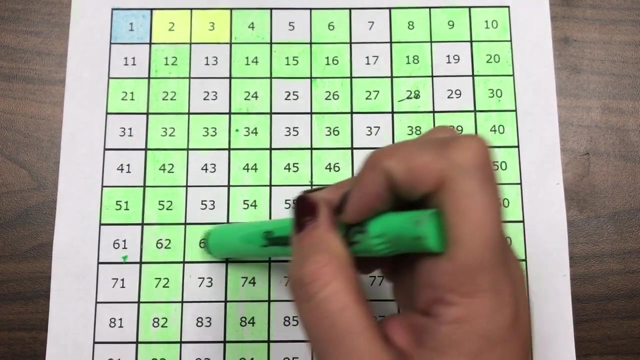 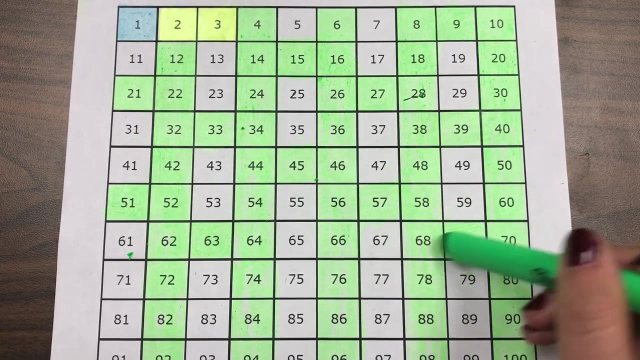 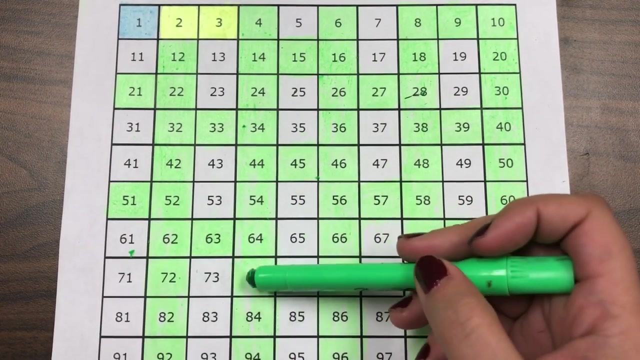 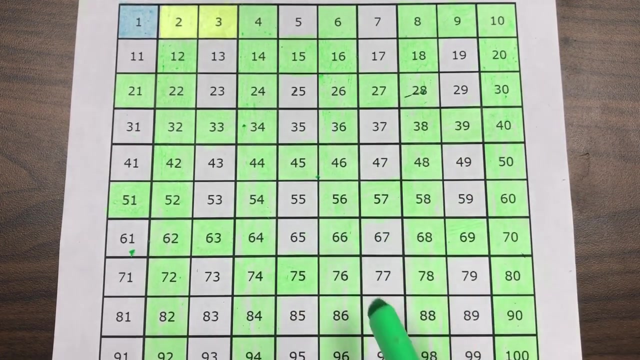 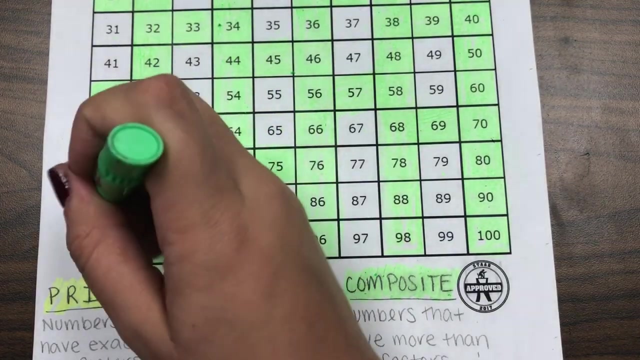 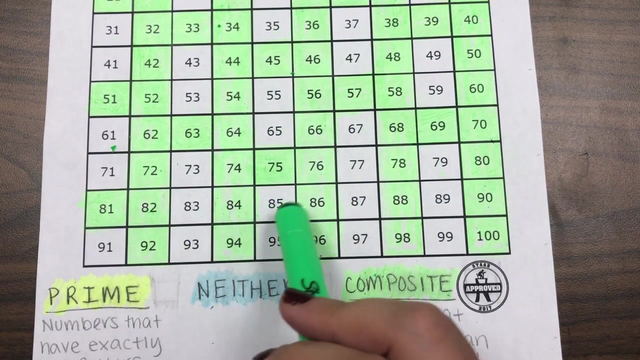 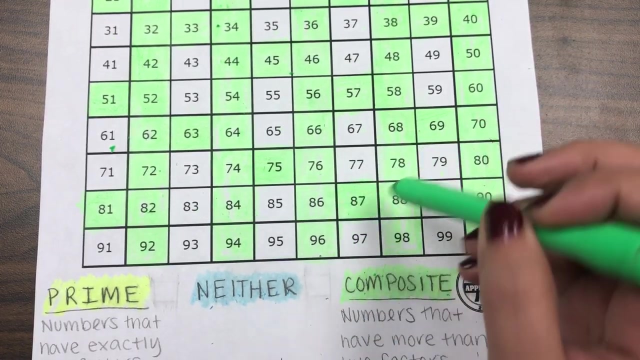 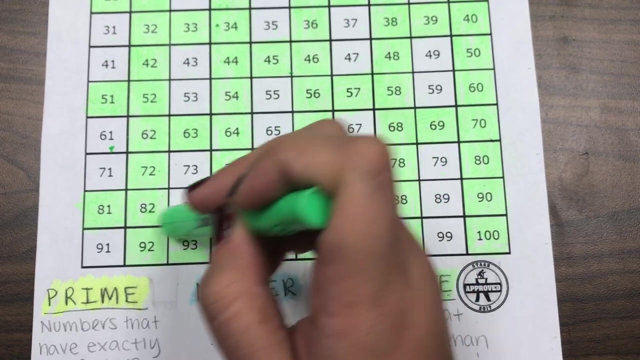 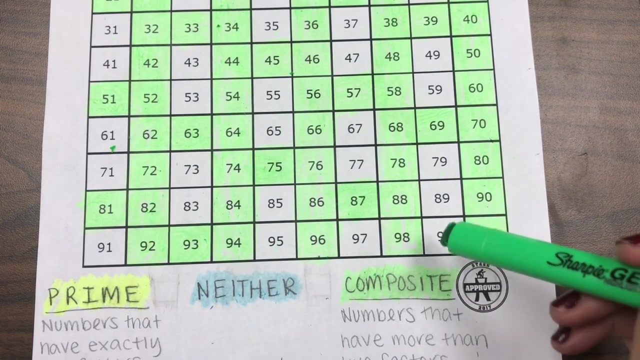 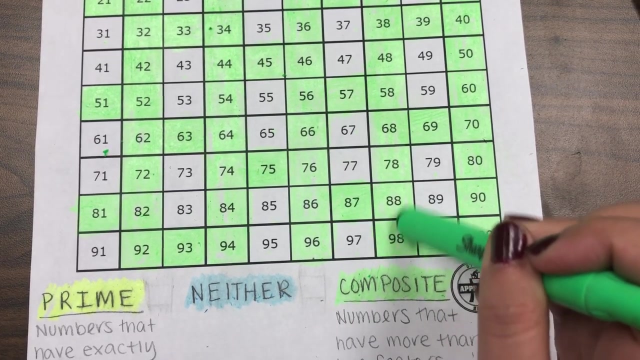 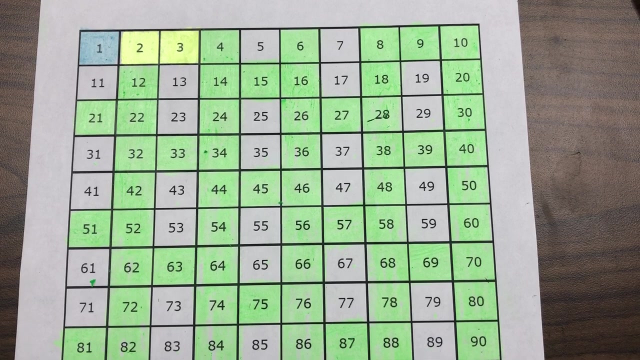 42, 45, 48, 51, 54, 57, 60, 63, 66, 69, 72, 75, 78, 81, 84, 87, 90, 93, 96, 99. okay, now let's go to the next prime number. the next prime number is five, so we're gonna. 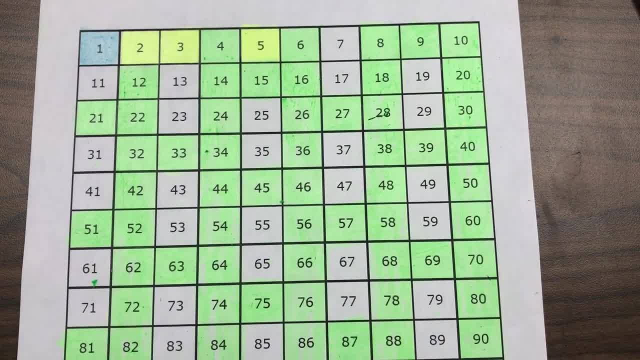 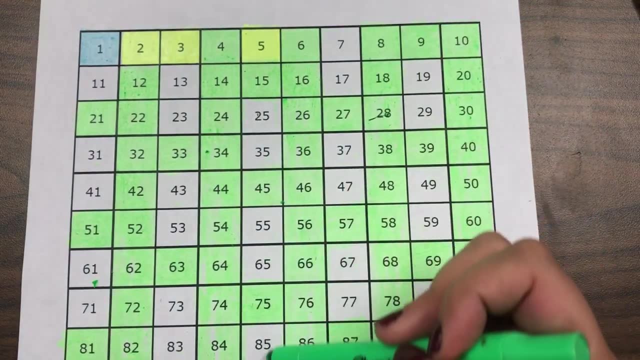 call her 15. we're gonna color that yellow. now. fives are easy because all the multiples of five have a five or a zero at the end. so, if you notice, all of the fives are right here. so we're gonna color this entire row. so we're gonna color this entire row. 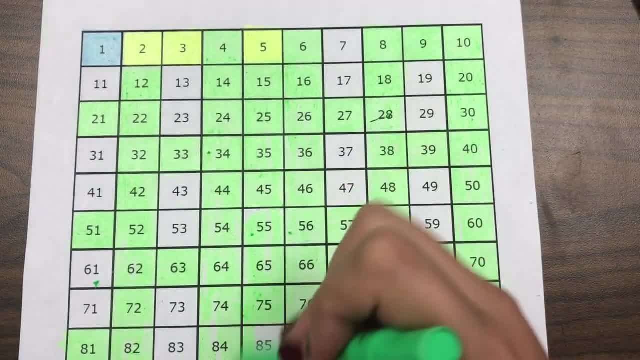 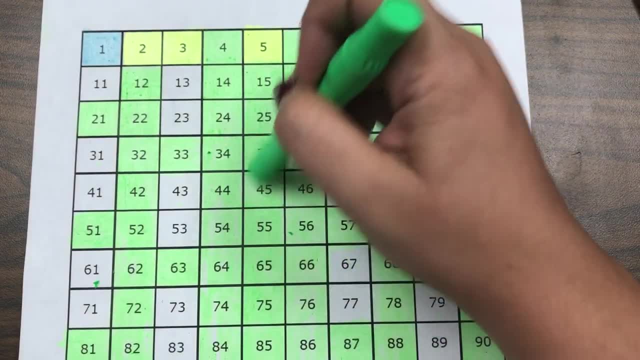 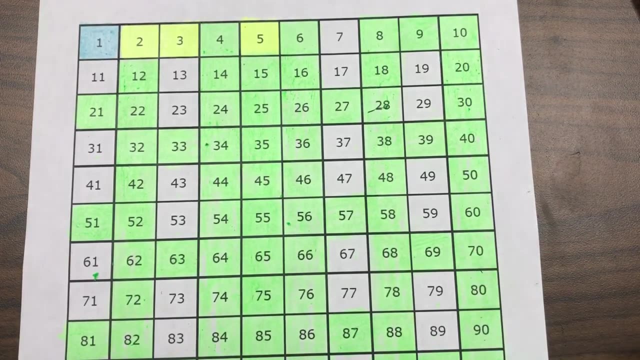 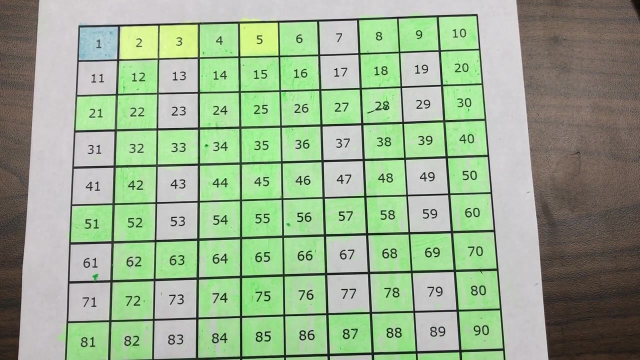 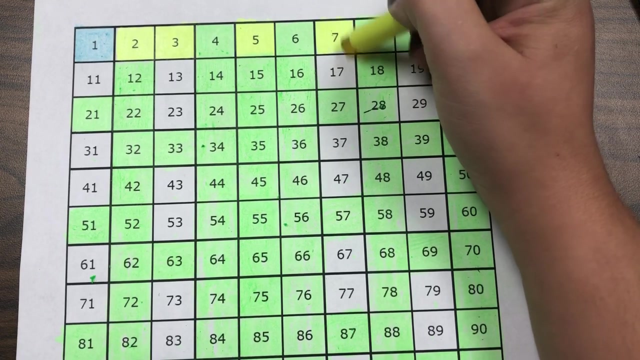 so we're gonna color this entire row. Now, all of the ones that have zero at the end are already colored, so we don't have to worry about those Now. the last prime number that we're going to color is seven. Now, this time we're going to count by sevens. 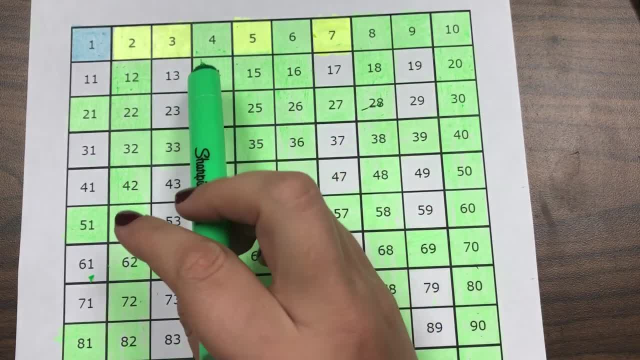 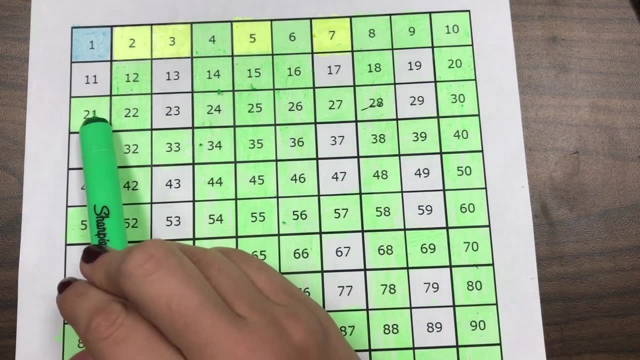 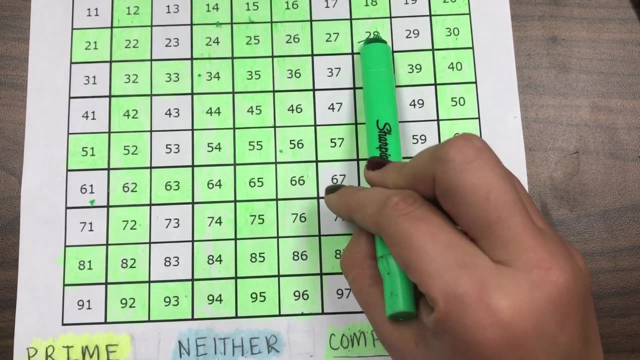 So seven, fourteen, it's already colored. one, two, three, four, five, six, seven, twenty-one is already colored. one, two, three, four, five, six, seven, twenty-eight is already colored. one, two, three, four, five, six, seven, thirty-one. 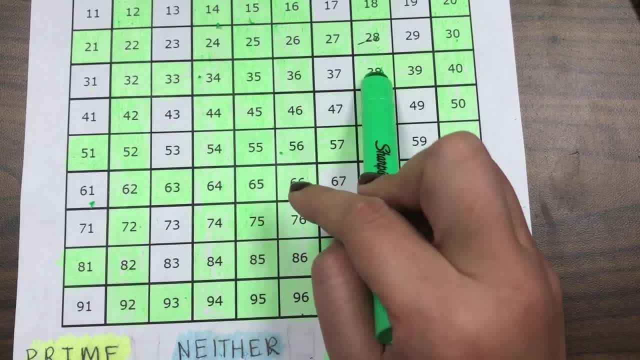 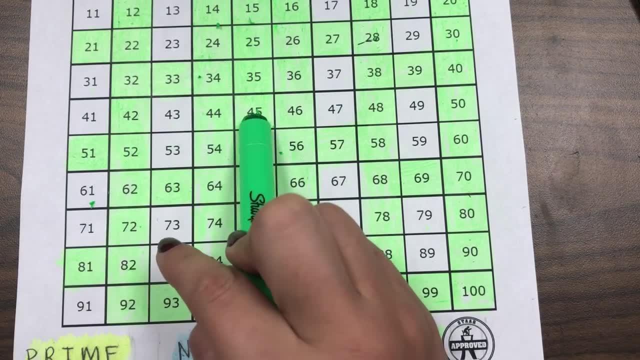 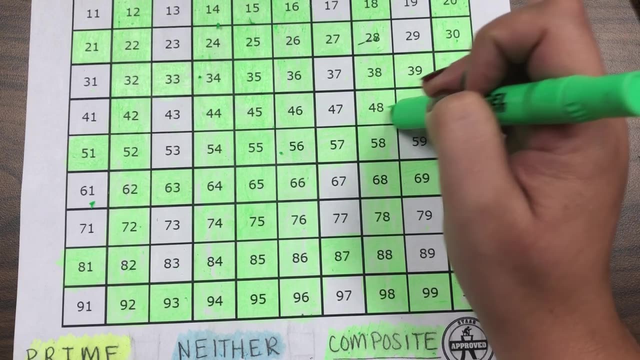 Forty-five is already colored: one, two, three, four, five, six, seven. forty-two is already colored: one, two, three, four, five, six, seven. Now forty-nine has not been colored, so we need to color that one. 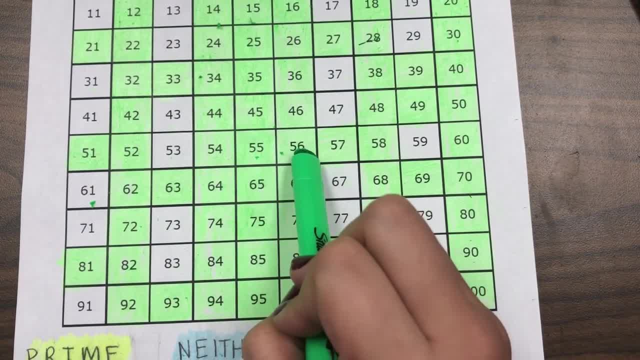 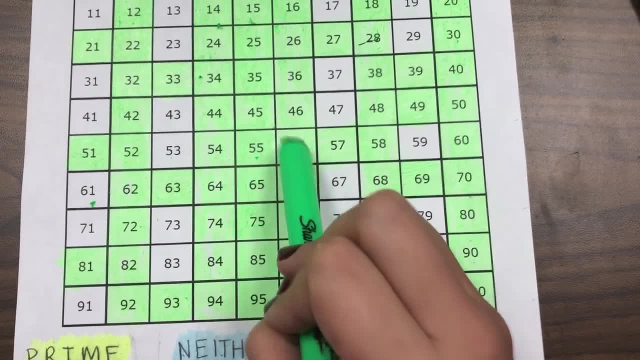 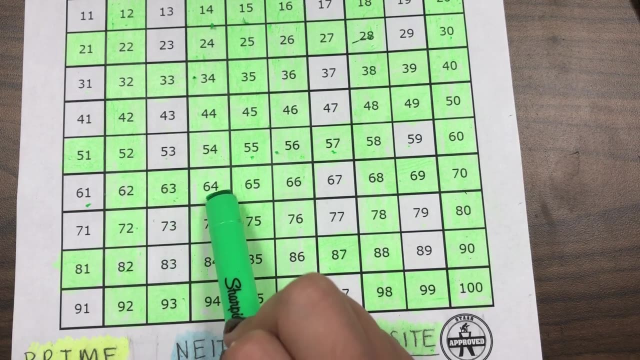 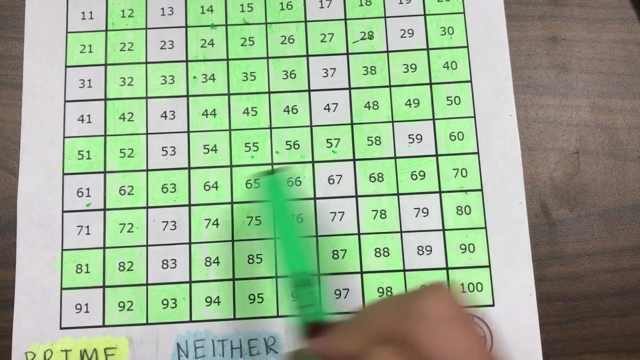 One, two, three, four, five, six, seven. Fifty-six is already colored. One, two, three, four, five, six, seven. sixty-three is already colored. one, two, three, four, five, six, seven, seventy is already colored. one, two, three, four, five. 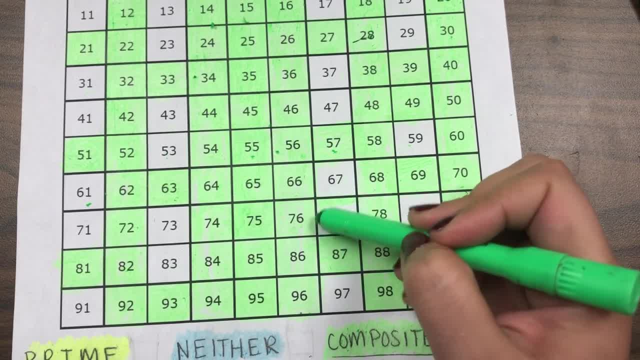 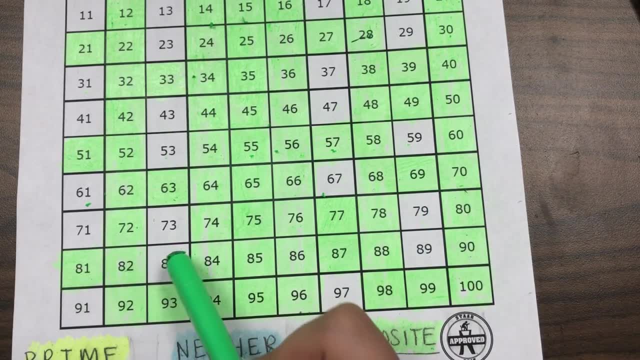 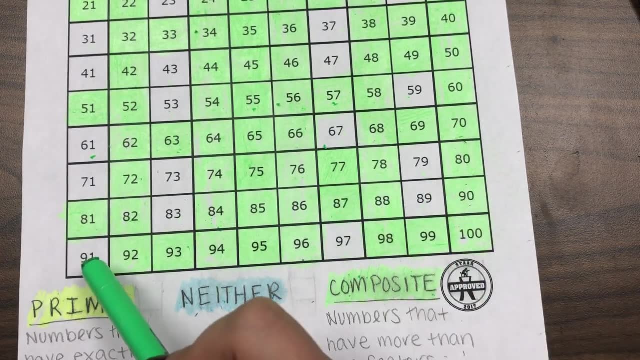 six, seven, seventy-seven has not been colored, so we're going to color that one. Okay, One, two, three, four, five, six, seven. eighty-four has already been colored. one, two, three, four, five, six, seven, ninety-one. 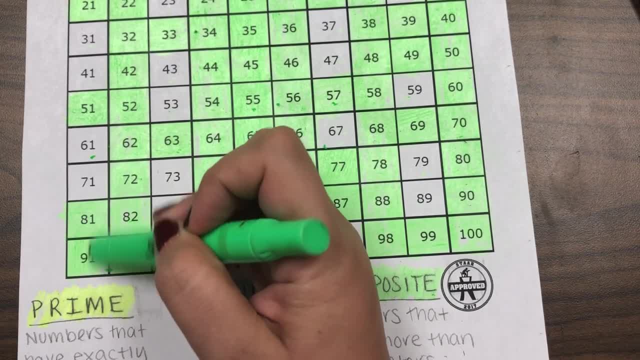 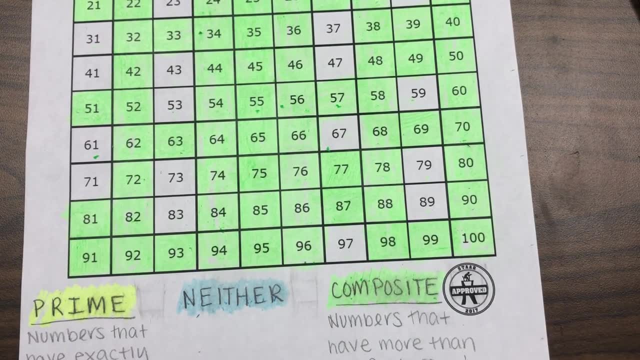 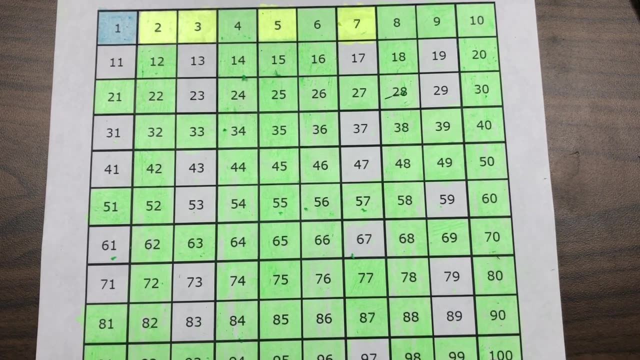 One, two, three, four, five, six, seven and that's it. So all of the numbers that are left over are your prime numbers. So I want you to get your units, Get your yellow, and we're going to color those yellows. 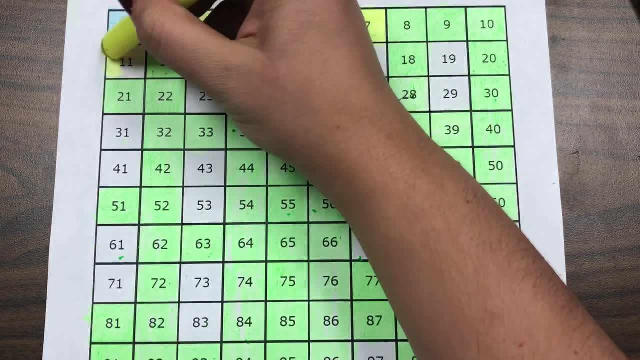 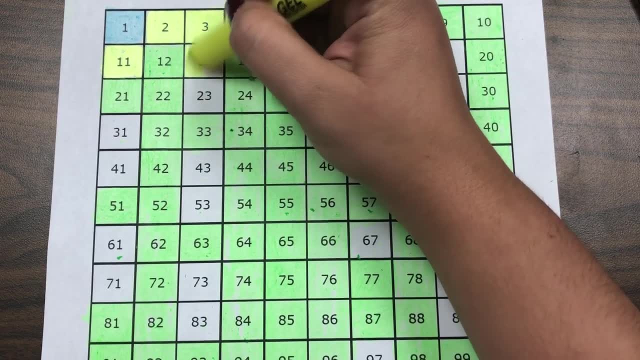 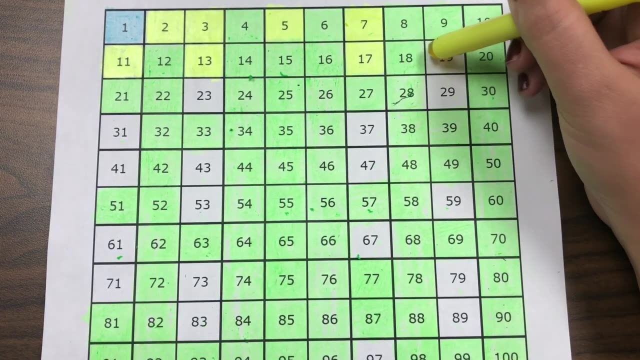 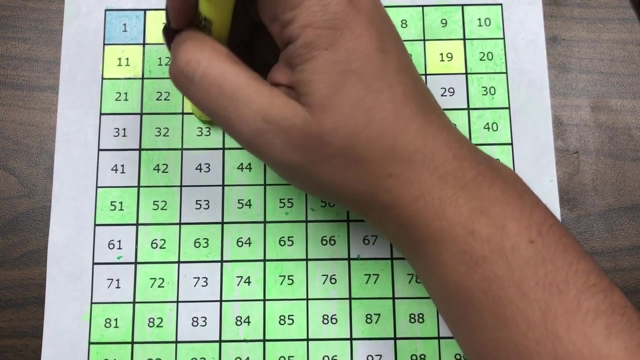 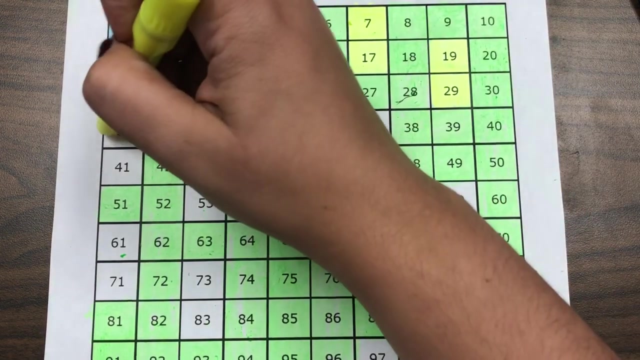 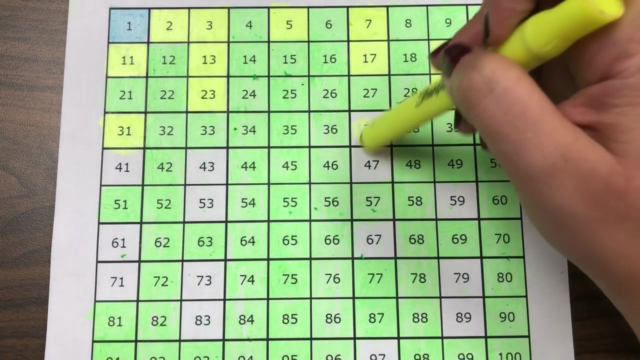 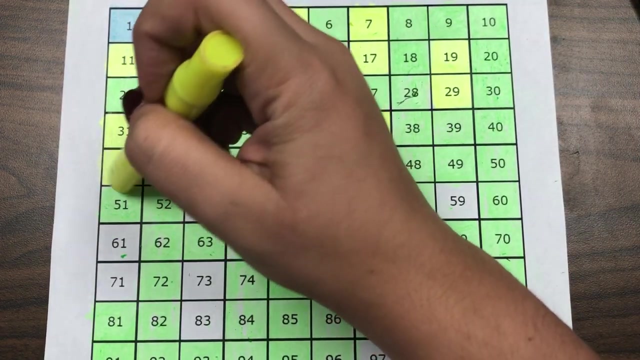 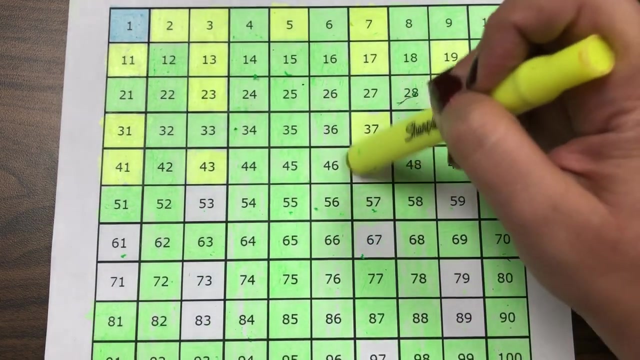 So two, three, five, seven, eleven, thirteen is prime, seventeen is prime, nineteen is prime, twenty-three is prime, Okay, Okay, Twenty-nine is prime, Thirty-one is prime, Thirty-seven, Forty-one, Forty-three. 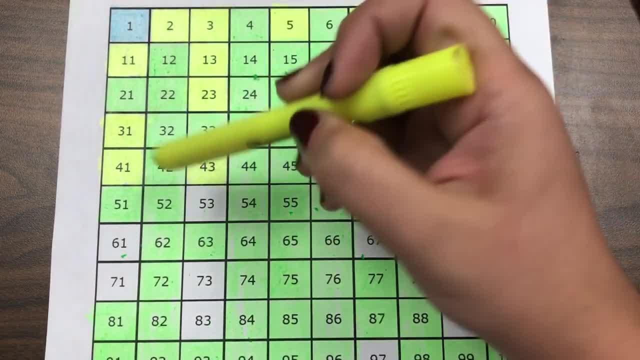 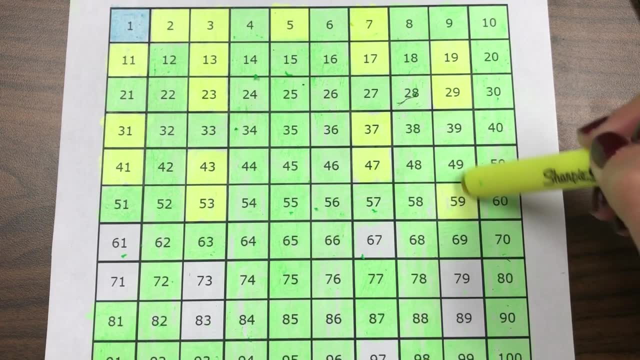 Forty-seven, Forty-eight, Forty-nine, Forty-nine, Fifty-three, Fifty-three, Fifty-nine, Fifty-nine, Sixty-one, Sixty-one, Sixty-seven, Sixty-seven, Seventy-one, Seventy-one, Seventy-three. 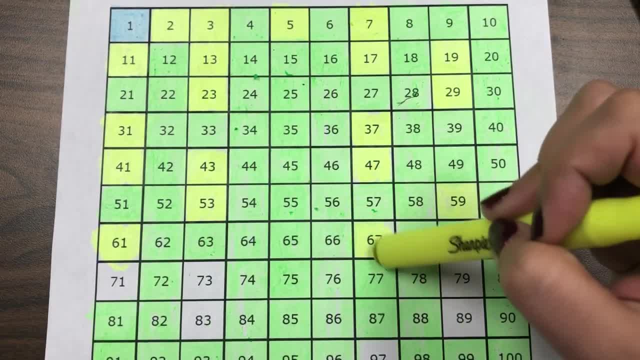 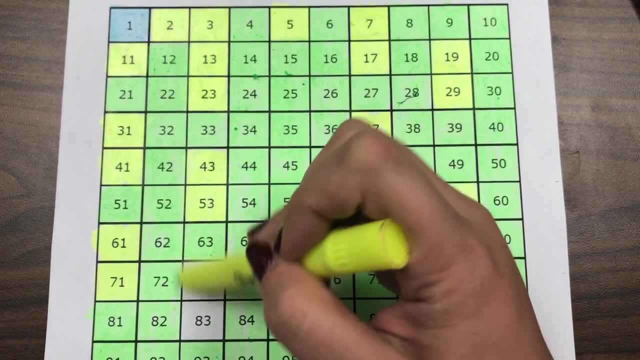 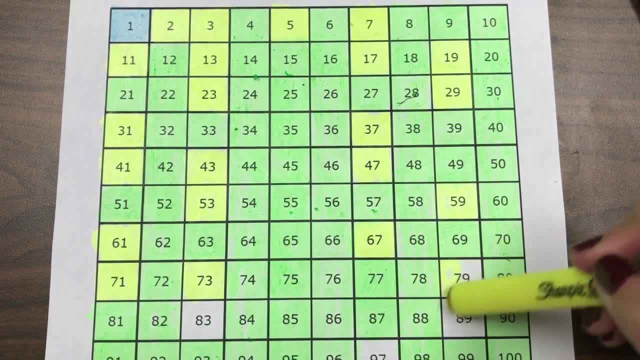 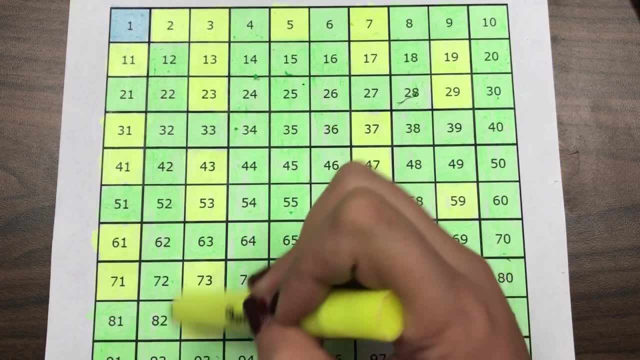 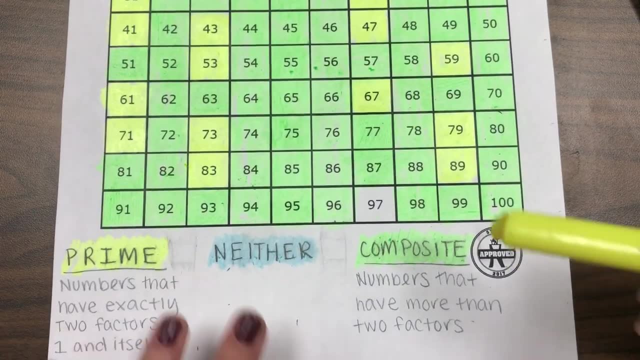 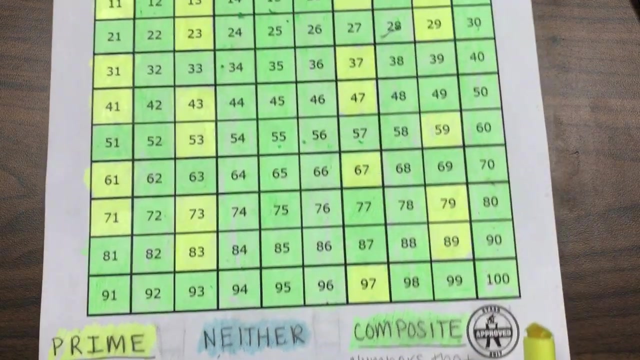 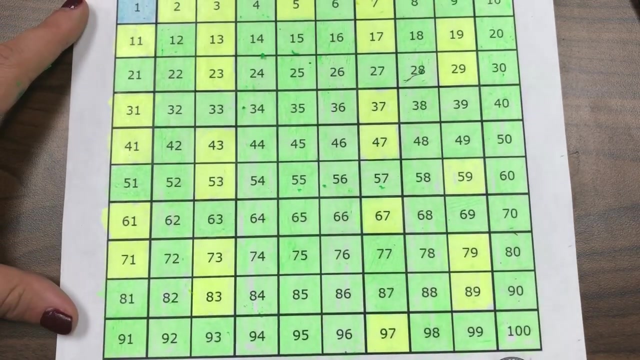 Seventy-nine, Seventy-nine, Seventy-nine, 83, 89, Finally 97.. So by going through all of the multiples of 2,, 3,, 5, and 7, you are able to find all of your prime numbers between 1 and 100.. 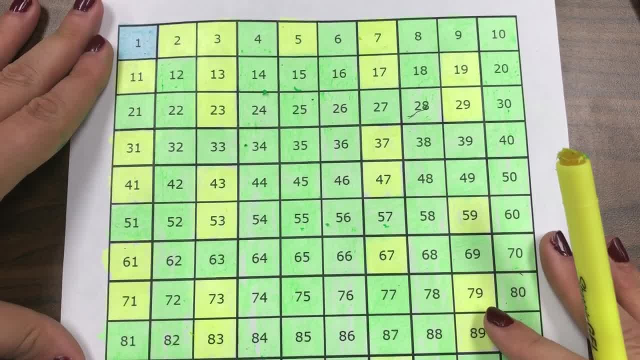 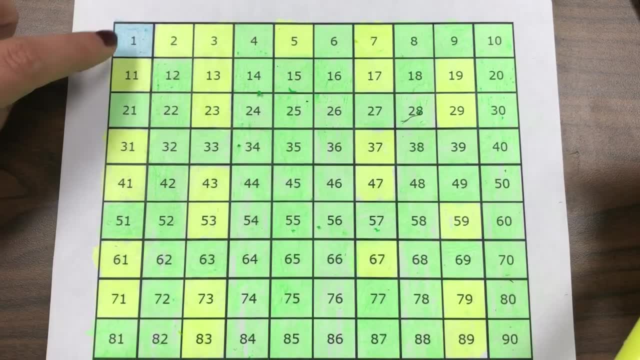 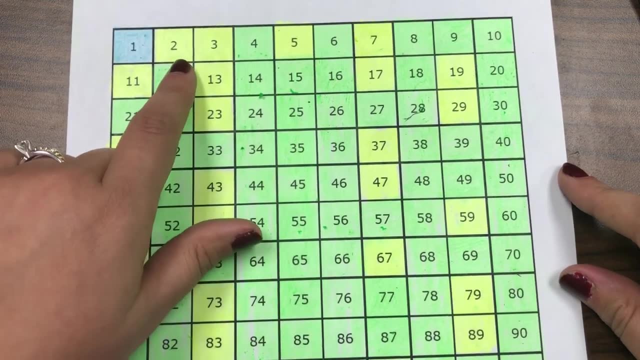 So now you can use this sheet as a reference to find your prime and composite numbers And remember the only number that's not prime and not composite is the number 1.. So I hope this was helpful. Remember your prime numbers.